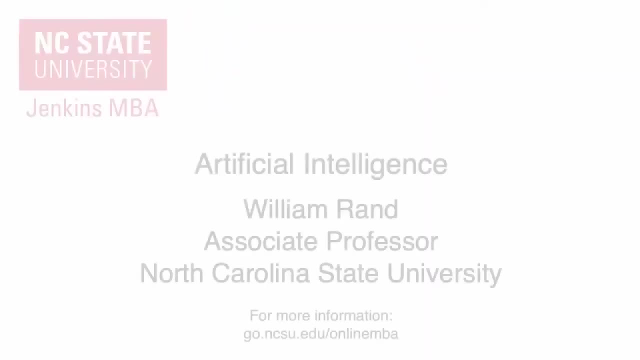 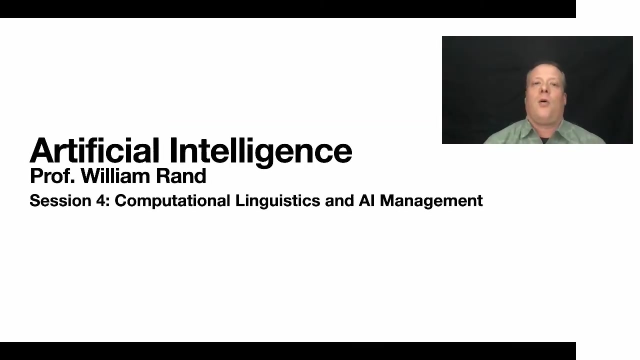 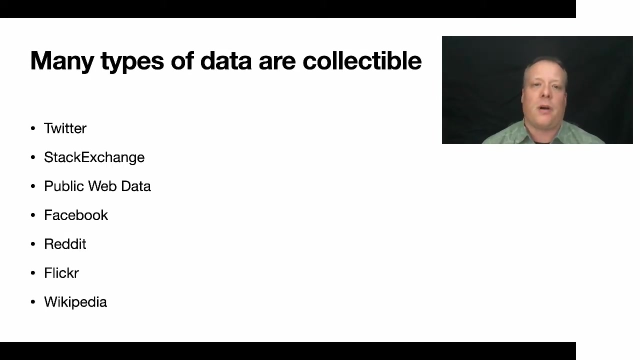 Hello everyone. In this section on artificial intelligence, we're going to be talking about computational linguistics, natural language processing and AI management. For this particular talk, I'm going to focus on using Twitter and doing natural language processing in that space. So why would you want to do what's sometimes called computational linguistics or 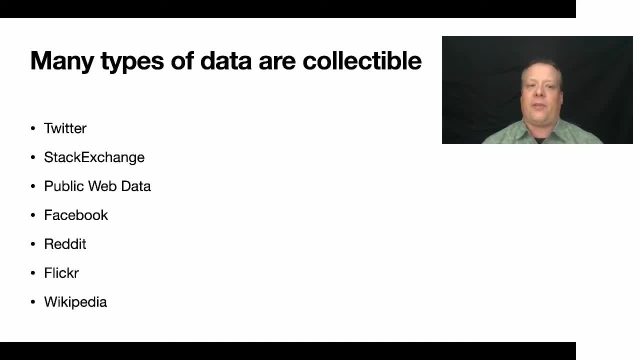 natural language processing. Well, there's a lot of data out there that's collectible. now that's in a language-based format that you really can't analyze via standard kind of regression analysis or something like that: Twitter data, for instance, or generally social media data. 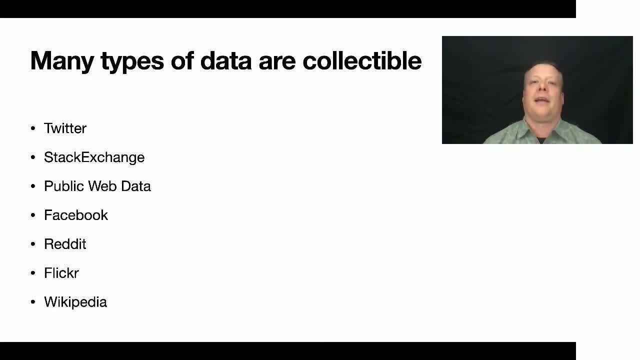 right Stack Exchange, which is this great repository of questions and answers, public web data about different companies and what they're doing, and things like that- Facebook data. right Now there's a lot of restrictions around Facebook data, but if you have public pages, that. 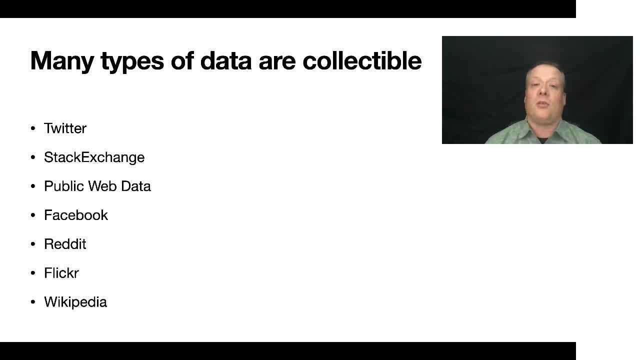 you can have your customers comment on that. data is owned by you to some extent. There's some different agreements on that, but you essentially can analyze the text that's there. Reddit is increasing in popularity. Flickr comments and hashtags right, And of course. 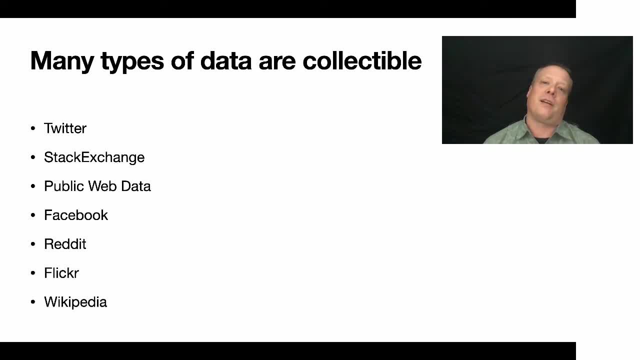 you could also think of Instagram, Instagram right And other photo sharing devices in the space, And in the next session we're going to talk about how to analyze the actual images, but today we're going to concentrate on the text that might be there And even like Wikipedia data right, So there might be data about different. 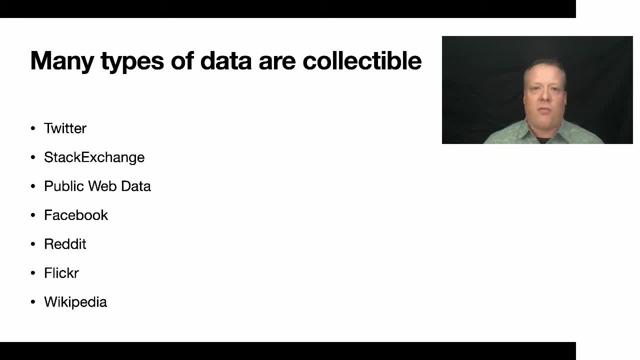 industries and about different aspects, and you want to watch how those things change and evolve over time, And, of course, this is just kind of things that are easily publicly available. You could also get into things like looking at the stock exchange filings right of major companies. 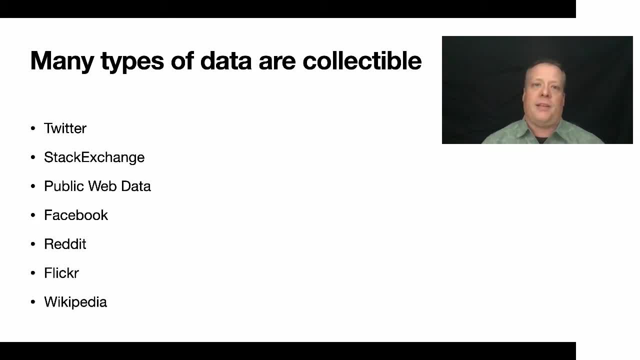 and using that to analyze the text that might be there. And of course, you could also get into things like looking at the stock exchange filings right of major companies and using that data to analyze where your company is doing in relationship to its competitors. 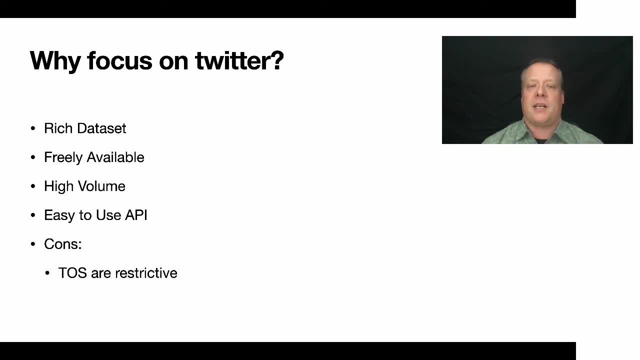 So we're going to focus, in this example and in this discussion, on Twitter. And why are we going to focus on Twitter? Well, it has a rich data set right. There's a lot of interesting aspects to it. It's freely available. it does take a little bit of effort to set up, and I'm going to show you. 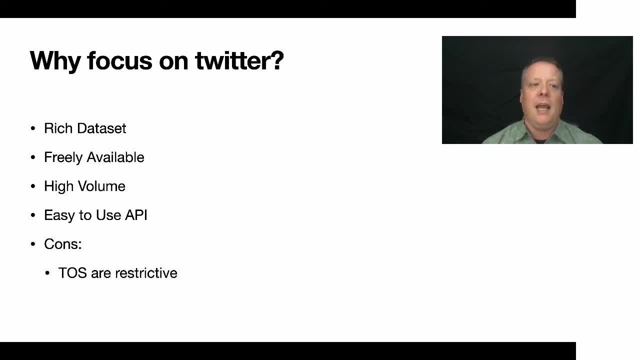 some tricks and tips to kind of get through that process easily. It's extremely high value So we can easily analyze it. I can in the session where I'm going to go through the R code. right, we can pull the code down and we can analyze, like literally, tweets that are being issued, right then. 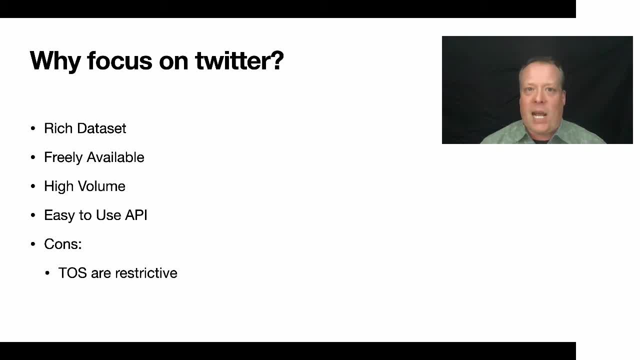 It has a very easy to use what's called an API or an applications program interface. This means that you can go out there and you can actually just request from Twitter certain amounts of data. Now, there's some restrictions on that and it's part of the cons, right. 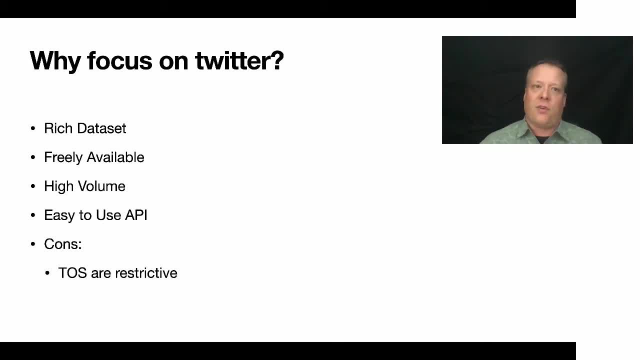 But you know, for instance, you can't collect historical data. that's too far into the past. Now there's tools out there where they can allow you to purchase that data or look at it, but it's not easily accessible. Another con is that the terms of service are somewhat restrictive. 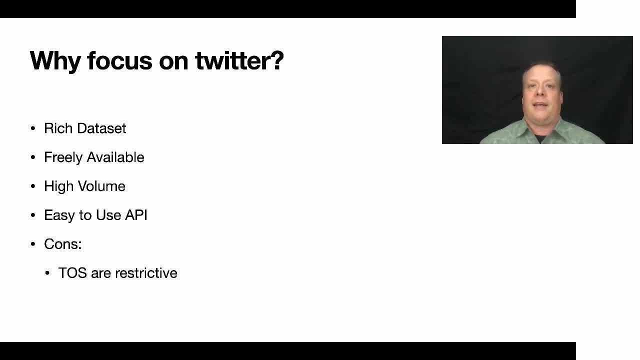 For instance, I can't just give you a bunch of Twitter data, right? I can't publish it on a website, I can't do a lot of things with it. I can use it for my own internal analysis and for my own internal examination. 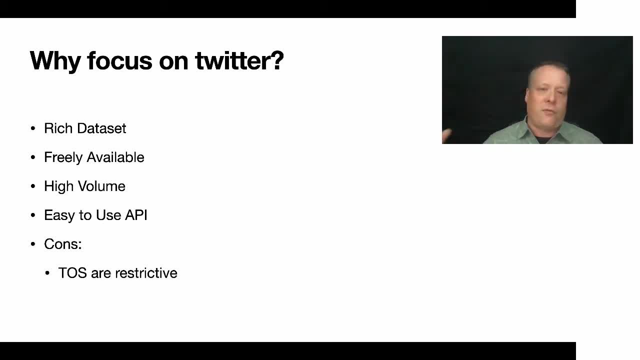 And that's pretty much about it right Now. if you have a group of analysts working together, you can share some Twitter uh data, as far as I know, Um, but you know you can't like republish that data and then make it available to someone. 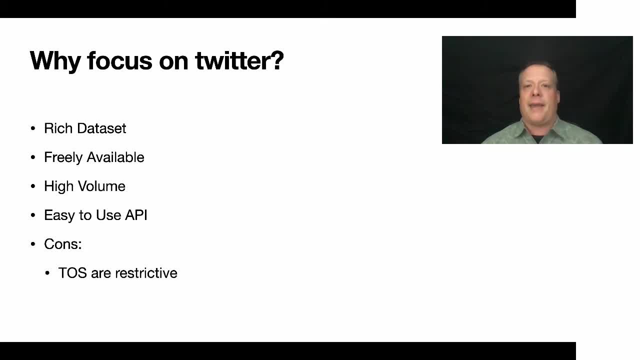 else, And there's also a lot of limitations on the API. You can only make so many requests per hour and things like that, But a lot of the tools that we're going to talk about actually take advantage of that for your deal with that situation automatically. 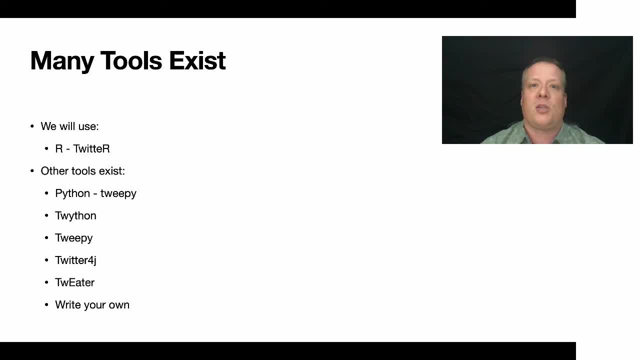 Um, many tools exist for Twitter data and for analyzing Twitter data. Uh, we're going to use ours uh, TwitR package uh, which is quite nice Uh, but other Other tools that existed in the past are things like: Python has Tweepy, there's Twython, there's. 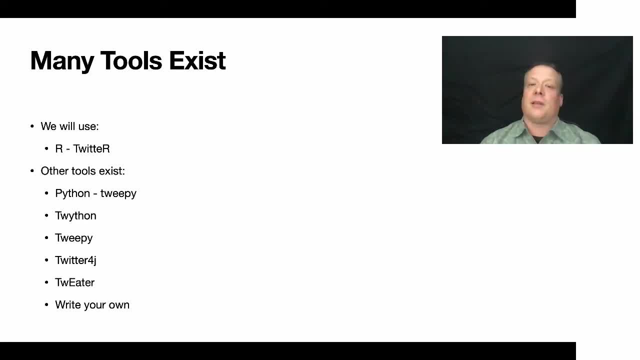 Tweepy, there's Twitter4j, right. Um, there's something called Tweeter, which I actually built early on in the uh Twitter years with a great grad student of mine named Derek Monard, which was, uh, it gave you the. 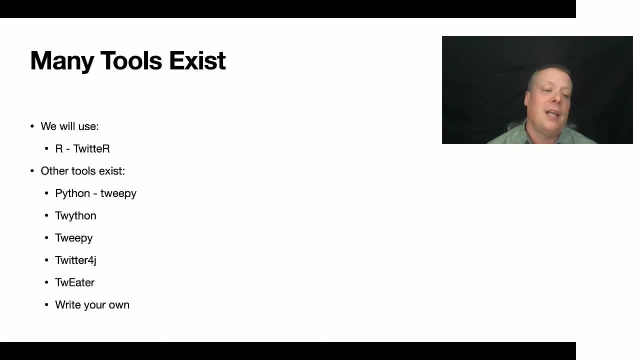 ability to pull down Twitter data in a systematic fashion. Uh, so there's a lot of tools out there. We're going to use TwitR because I try and do all this class in one platform and just do it in R, basically, And the API is. 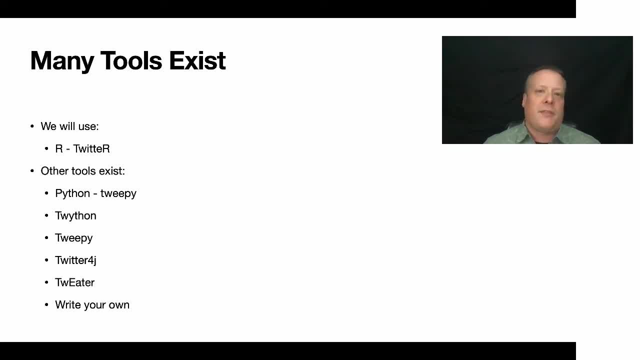 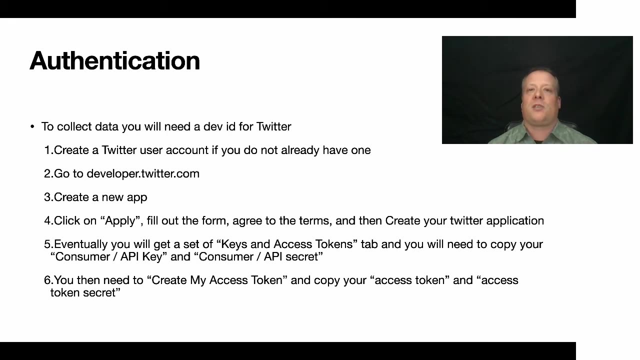 Publicly accessible right. It's well documented. If you're a sufficient enough programmer in R or Python or Java C or any language, you can actually create, uh- your own Twitter data collection tool. So one of the things you need to do in order to use these tools, though, is in order you 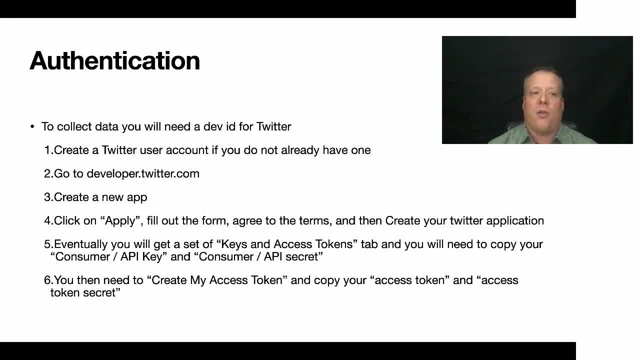 need to have a developer ID for Twitter. Um, so the first step of that is that if you don't have a Twitter user account, you need to create one right. Then, once you have your account, you can go to developertwittercom. 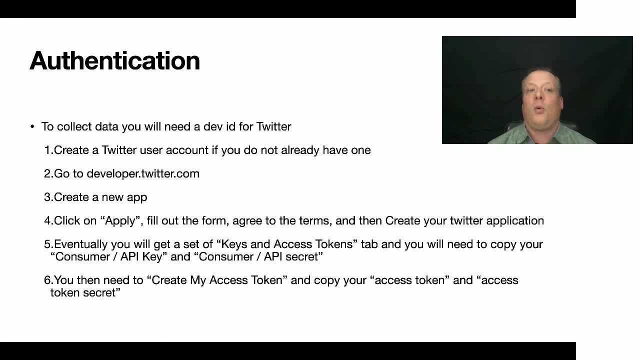 And there's an app law application process you have to go through to apply for the dev ID. Um, I don't have the exact details here because it kind of changes on a regular basis. Uh, but basically, once you fill out this form, you're going to set in green to the terms. 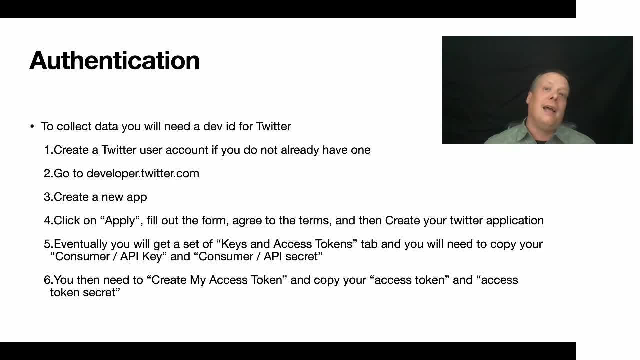 you're going to set it up, you send it off and Twitter's going to look at it and they're going to decide whether or not to authorize a dev ID for you, Right? Um, as far as I know, no one I know has ever been denied one. 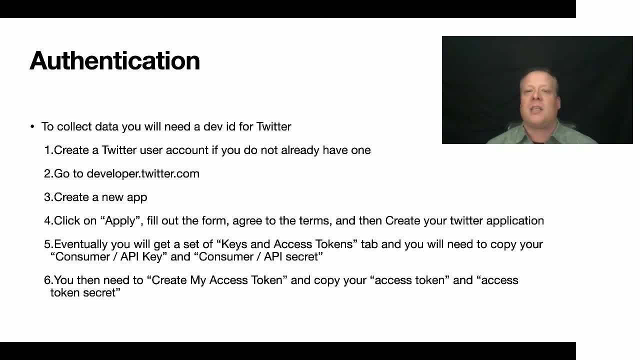 There have been follow-up questions Sometimes where they've set back questions a lot of times. if you tell them you're working on the class project, from what I understand, they're a little more lenient about it. Um, but, um, they, um. they will sometimes ask questions and it may take three or four. 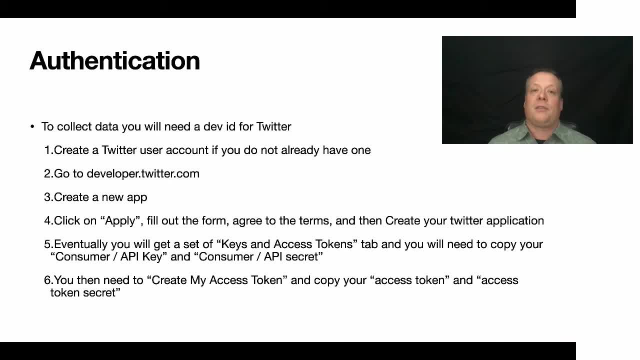 days for you to get that dev ID created. So if you're going to use it for the class project here, I would recommend doing this almost immediately after watching this video. um, eventually you're going to get access to the developer platform and you should see a set of keys and access tokens tab. 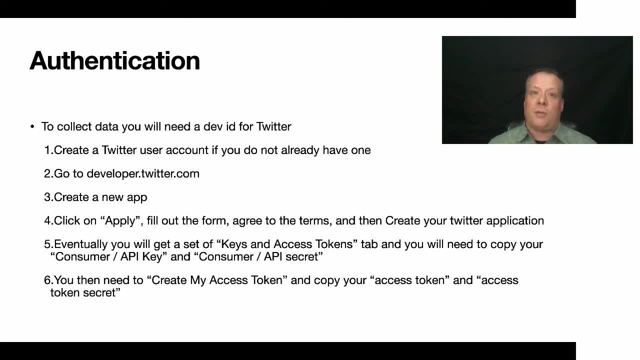 Yeah, Um, and you'll need to copy your consumer API key and consumer API secret. Um, you also need to create an access token and use your access token- access token secret- to access, uh, Twitter. I'm going to pause here. 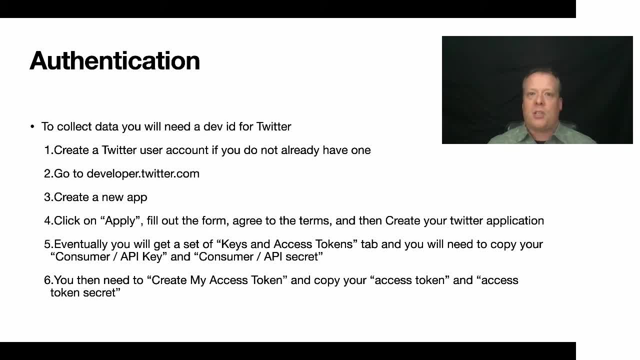 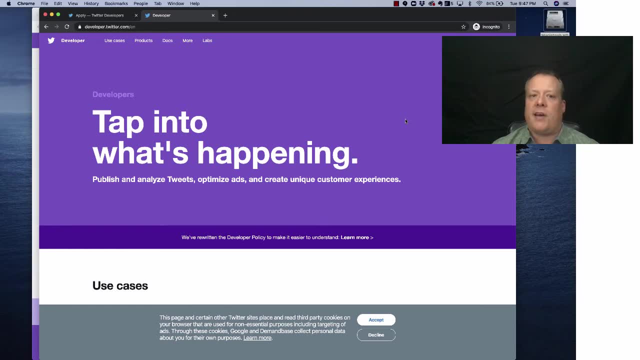 I'm going to flip over to the actual Twitter dev ID page So I can show you a little bit of this Um, and then I can show you what it looks like once you have the developer accounts as well. Okay, Okay. So I'm going to take you through a little bit of the process of how to apply for. 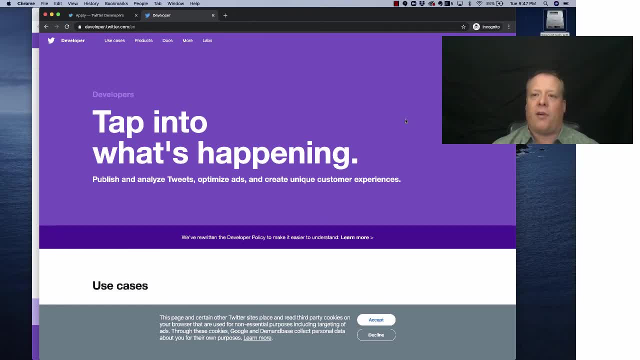 a developer account. So, um, if I want to divide apply for an account, I first have to log in, and I'm not going to use my normal Twitter handle, I'm going to use one that I manage for a journal. Uh, but, um, I hit the apply button once I'm logged in. 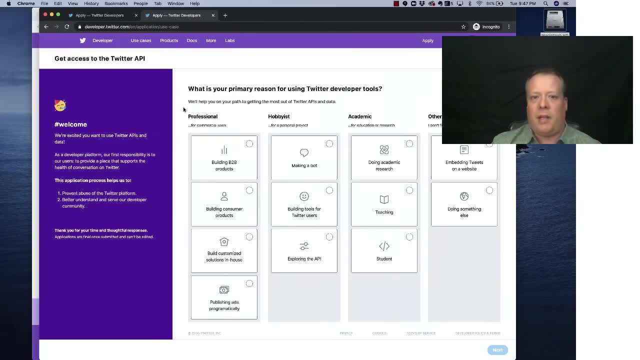 If you haven't logged in, it'll say: you know, log in, um, and I'll go to apply for an academic account and wants to know the reason why, Um, and you know, ideally for this, if I was really doing it for this academic. 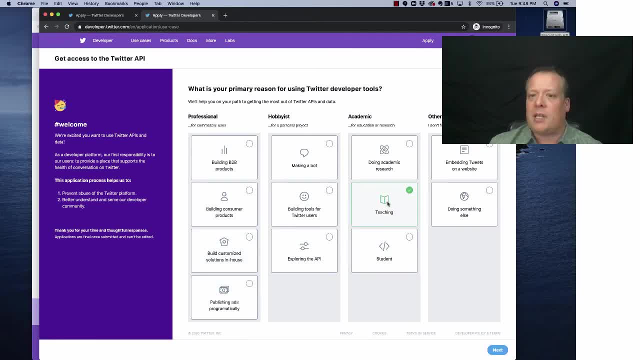 journal. I'd probably be like building a customized solution house, But right now I'm just going to click the teaching button, Cause that's what I'm doing right now. Um, you could probably click students, right, And then it makes sure that you have some information. 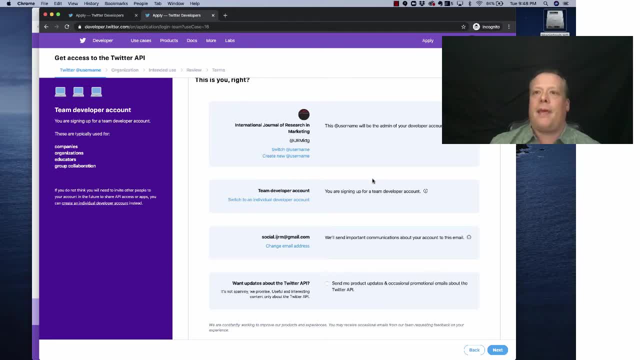 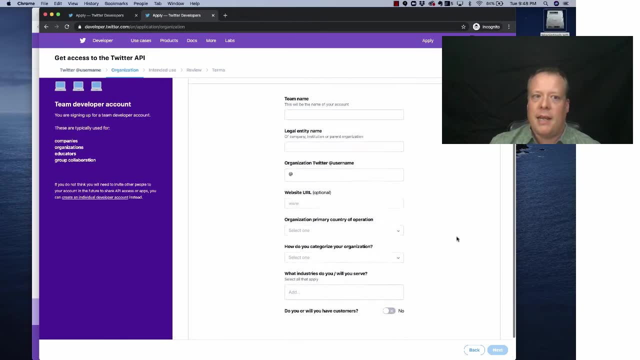 If you don't have a um, A phone number entered, you'll have to enter that, And there's some other details along those lines. but eventually you hit click next. And now I have to say, like what? who is the organization? 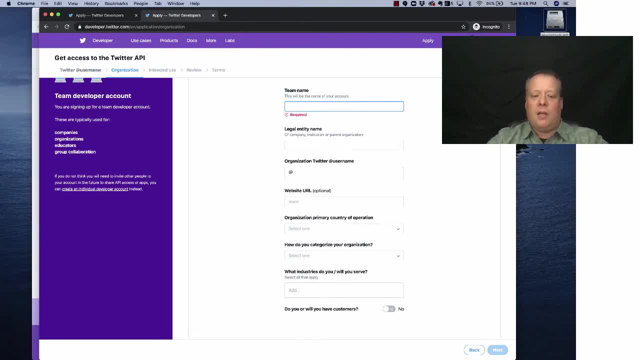 And I can say like, um, um, you know, let's just I'll full, I'm not going to complete this application, but I'll just do full college, right, NC state University. Right, I um at, say at the organization name, which probably at pool. 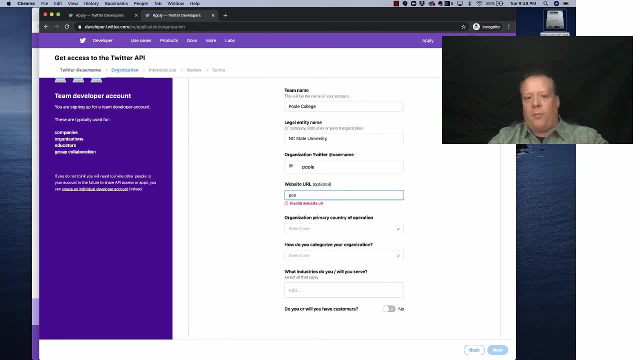 Um, I don't know for sure, Right, Um, you could go poolncsuedu. uh, primary country of organization is going to be United States. How do you characterize your academic? um, and then, uh, academic, right. 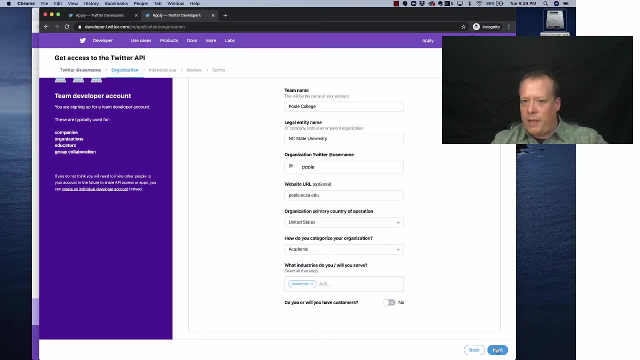 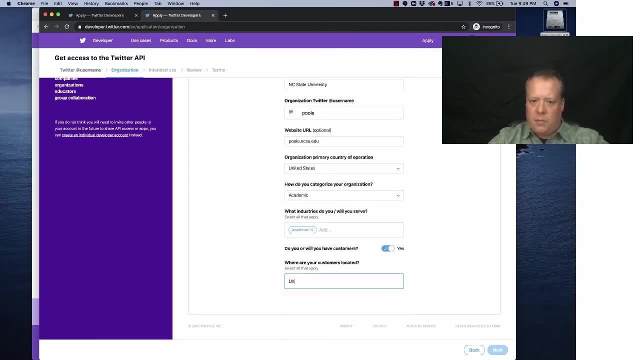 So we'll just say we're Academic, um, we don't have. I mean, let's say we have customers, right, And those customers are also located in the United States. Oh, it has to be specific: North America, Okay. 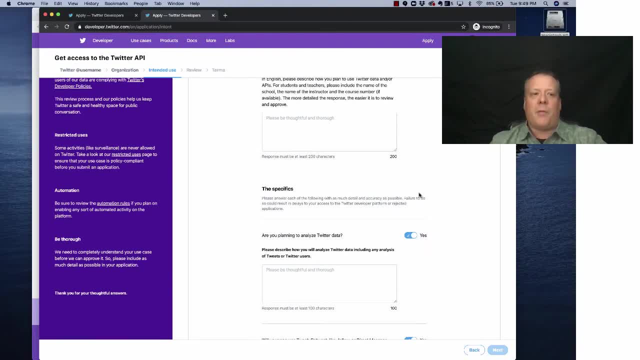 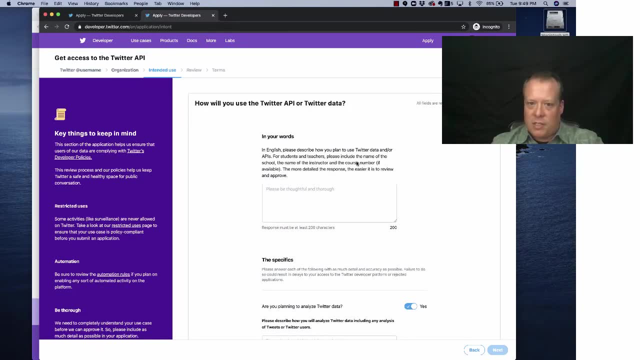 So then I hit next, And then this is the part where I'm going to kind of stop, because this is the part where it gets a little detailed, but you essentially have to write why you want to use it. and see it says: for students and teachers. please include the name of the. 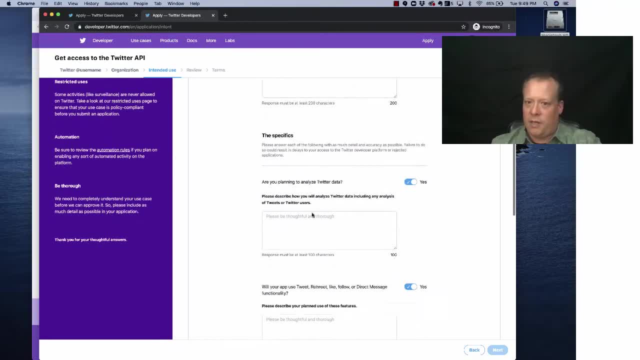 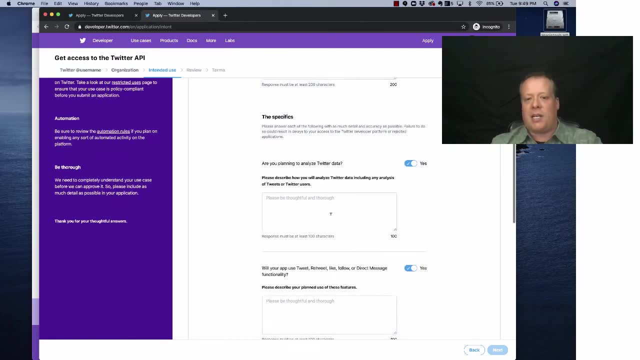 school name and structure in the course number. So you put my information down there, if you want to do that. Um, please describe how you analyze. for us is primarily going to be like sentiment analysis for a class project, but you can put down whatever you want. 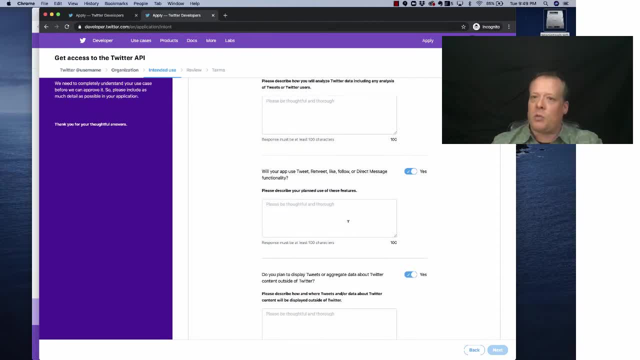 We're at use tweet retweet like follow direct. probably not Right, Because we're just going to collect the data. Uh, do you plan to display tweets or aggregate data about Twitter content? And the answer is yes? 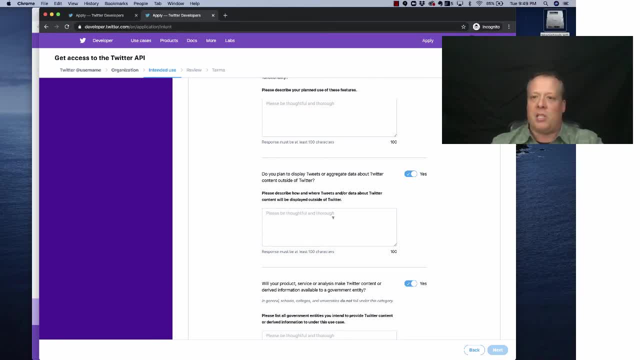 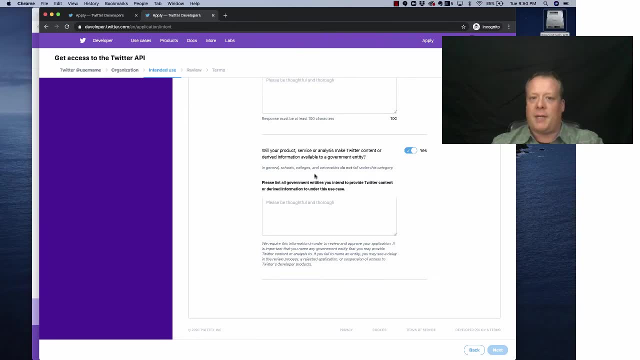 Right, You're going to be looking at the content, but you're not going to republish it or present it anywhere else besides inside this class. So make sure you note that. uh, will your product service make Twitter content or drive information? 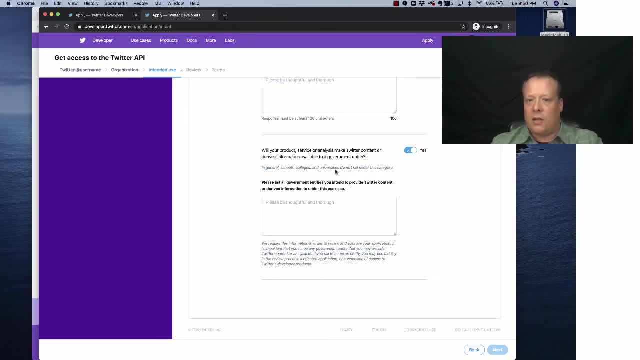 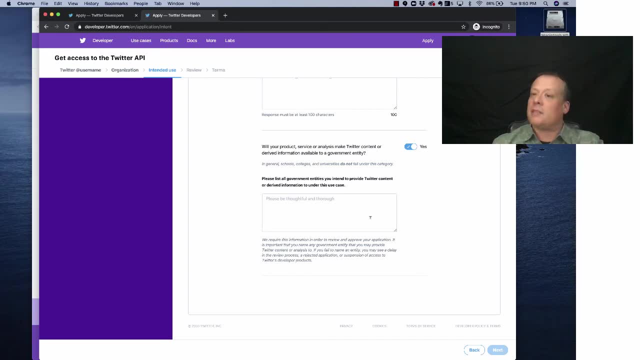 You can be able to a government entity, Um, and as it says, you know, universities do not fall under this category. What they're specifically talking about is if you were going to use it, uh, for a public policy type process at like a regional government or something like that. 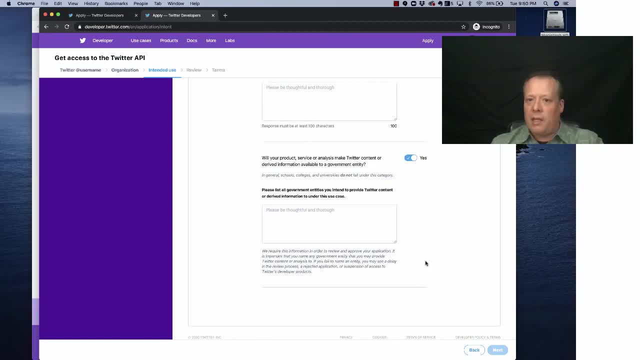 Right, So I'm going to stop there. I'm not going to flip over again and show you what the account looks like once you've done, once you've got it. Um, so, as you can see, you need to review it, agree to some terms and then you'd. 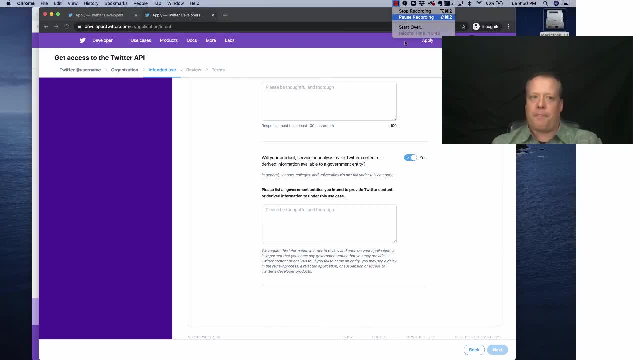 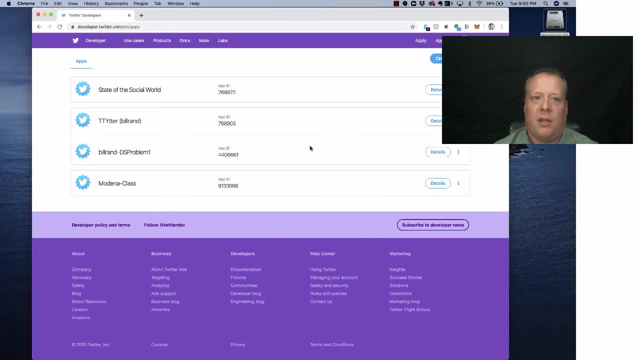 have, um, your account be monitored, Okay, So here's what it looks like once we actually have an account. and this is my actual account, So it has all the the information up there, Um, uh, I'm going to click on one of these. 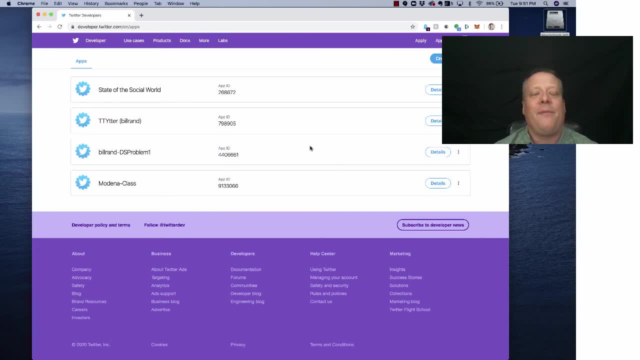 I'm not going to click on all of them, because I use some of these still. Uh, but I have. you can apply for different apps for different purposes, right? And each of them will actually present you with uh, the uh, its own app ID and its. 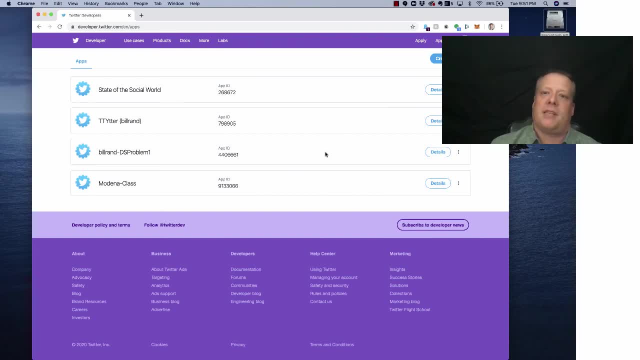 own authentication scheme, So you can have multiple apps, uh with the same developer, Uh, but the most important part is, if you click on the detail, Um, and this is uh the first one I think I ever created, right. 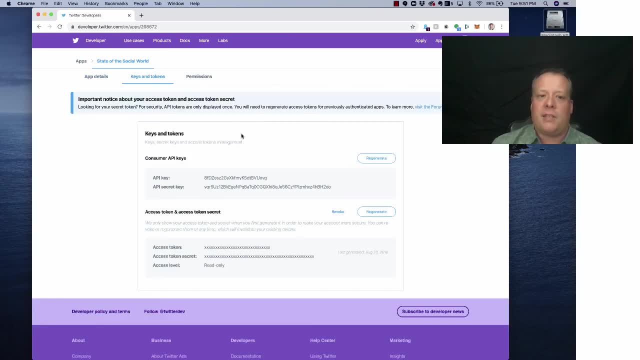 Um, and you go over to keys and tokens. These are the numbers you're going to need that. we talked about the access keys, Right? Um, and yes, I'm showing you my consumer API keys right now, but as soon as I save. 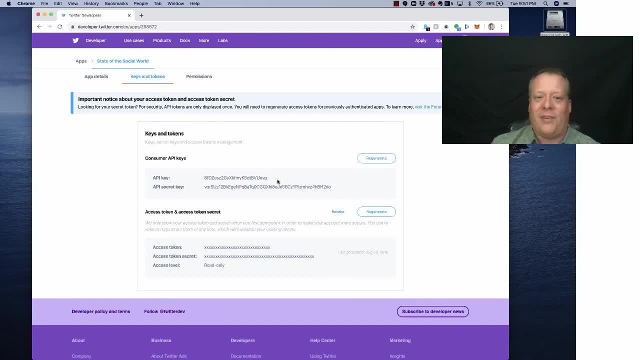 this video. I'm going to regenerate them so they won't be useful, So don't bother trying to keep them down. I'm not going to show you the access tokens, right, But all these data is what you're going to need to actually run with the R script. 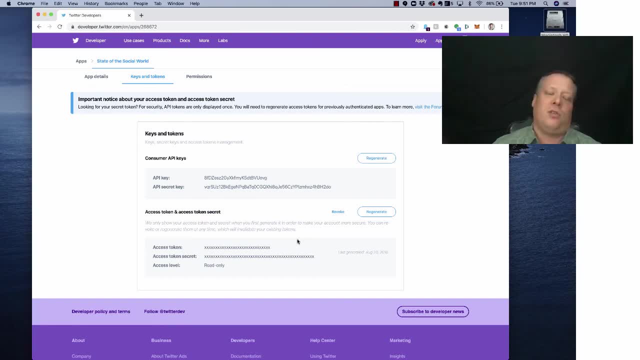 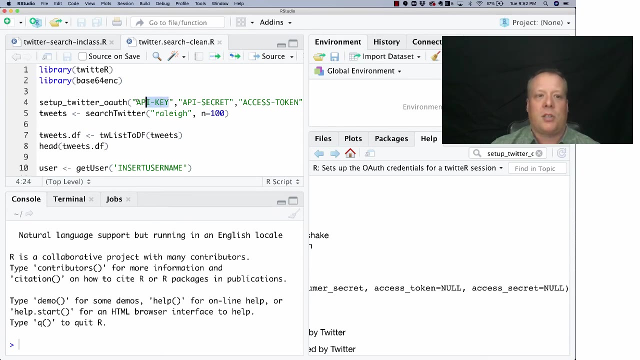 And I'm going to do a separate whole video About how to actually pull the data with our. once you have this by, I'm going to flip over quickly to just show you where to paste these numbers in. Okay, So here we are, back in, uh, our studio, and you'll see that there is this Twitter. 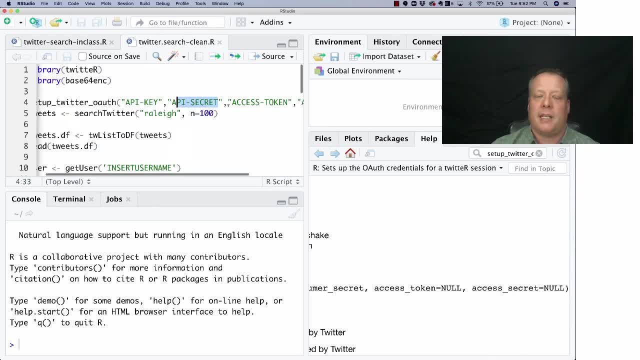 setup where you're going to piece in those API keys and secrets- And I made this code available to you on the Moodle- and then the access token and the access secret, right, Um. so that's where you would put in those uh strings that you.